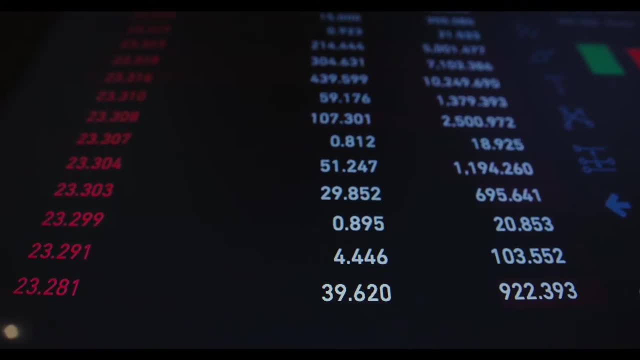 crimes like identity theft, fraud or fraudulent activity. A man-in-the-middle attack is a man-in-the-middle attack in which an attacker intercepts an ongoing conversation or data transfer by eavesdropping or posing as a legitimate participant. Because man-in-the-middle attacks are carried out in real time. 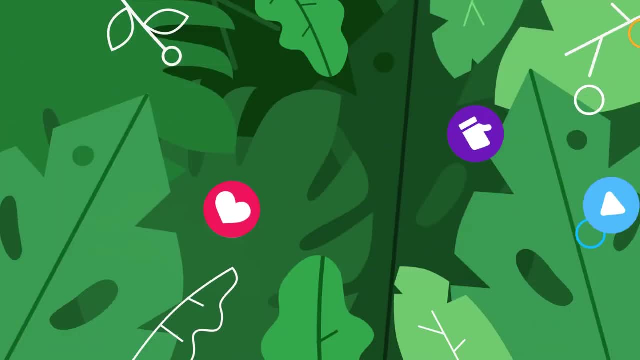 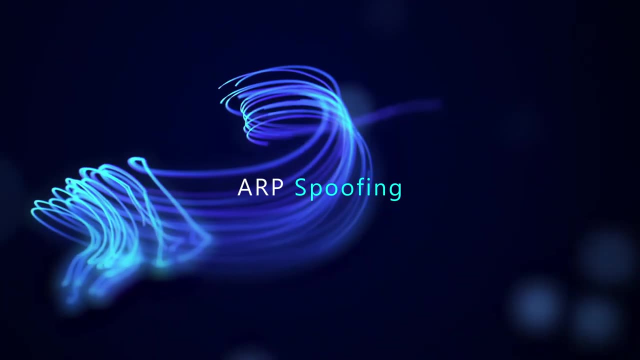 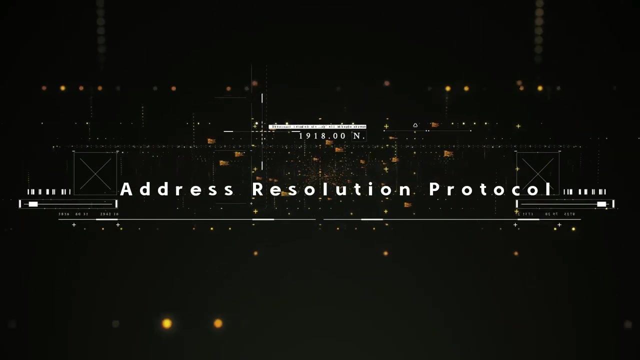 they often go undetected until it's too late. Now let's look types of man-in-the-middle attacks. The first is a RP spoofing. RP is the address resolution protocol. It is used to resolve IP addresses to physical 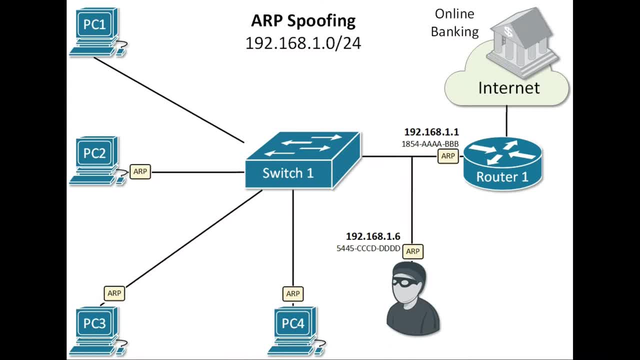 MAC addresses in a local area network, When a host needs to talk to a host with a given IP address, it references the address resolution protocol cache to resolve the IP address to a MAC address. If the address is not known, a request is made asking for the MAC address of the device with. 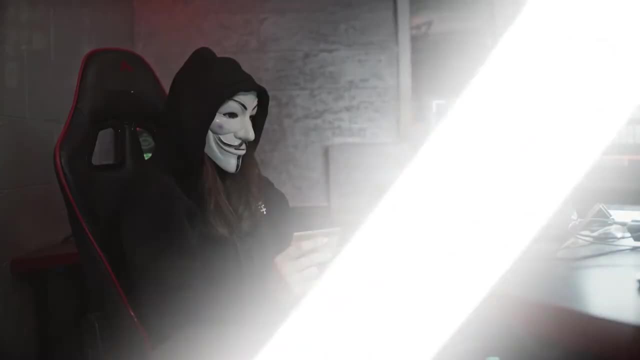 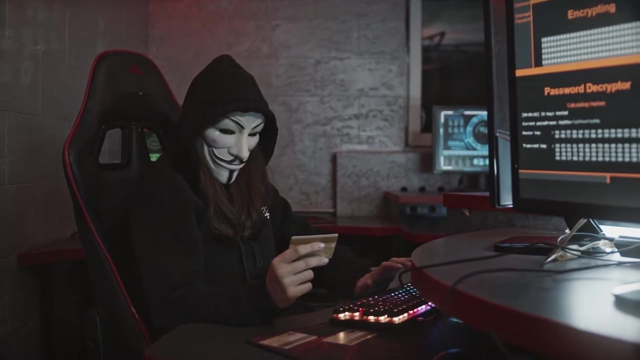 the IP address An attacker wishing to pose as another host could respond to requests it should not be responding to with its own MAC address. With some precisely placed packets, an attacker can sniff the private traffic between two hosts. Valuable information can be extracted from the 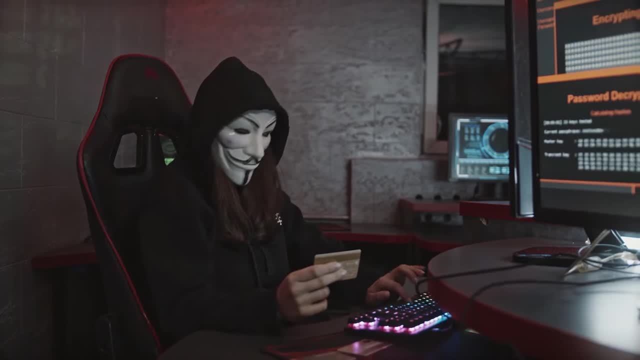 traffic, such as the exchange of session tokens. An attacker can sniff the private traffic between two hosts. Valuable information can be extracted from the traffic, such as the exchange of session tokens Yielding full access to application accounts that the attacker should not be able to. 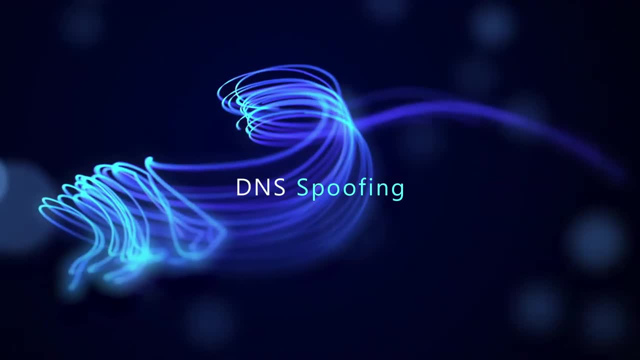 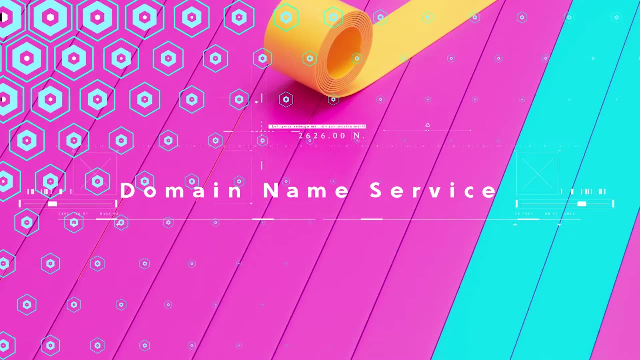 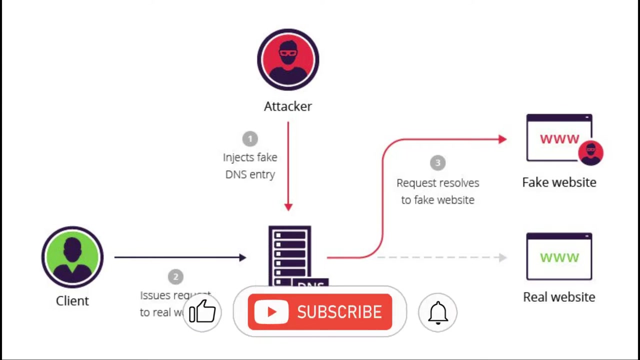 access. The second is DNS spoofing. DNS or domain name service spoofing is the process of poisoning entries on a DNS server to redirect a targeted user to a malicious website under attacker control. The DNS attack typically happens in a public Wi-Fi environment. 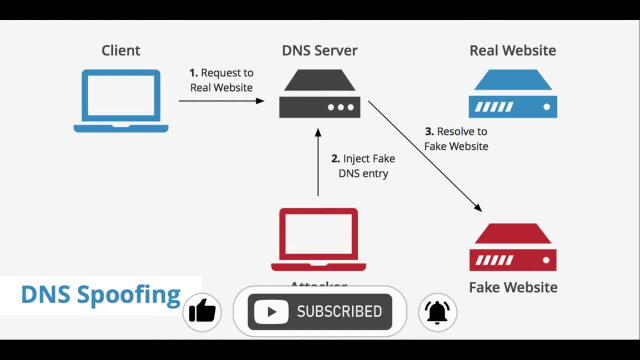 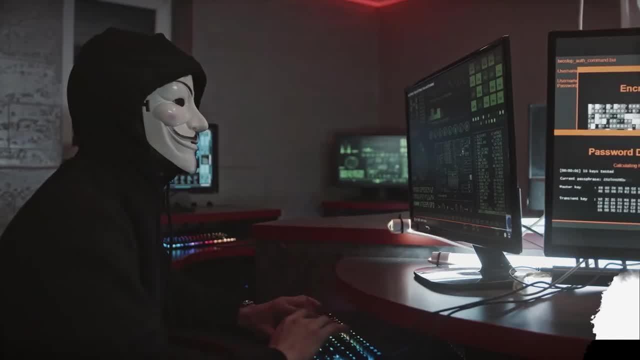 but can occur in any situation where the attacker can poison tables and force targeted user devices using the attacker-controlled machine as the server for a specific website. It's the first step in a sophisticated phishing attack on public Wi-Fi, and it can also trick users. 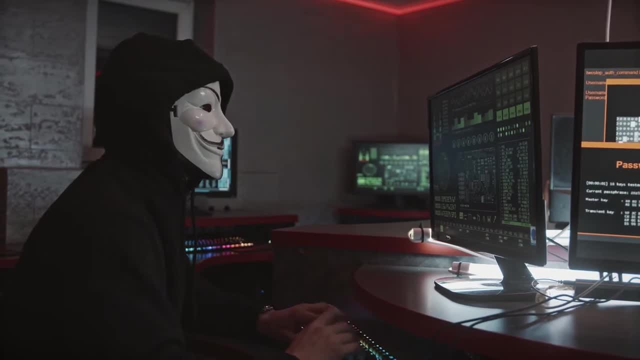 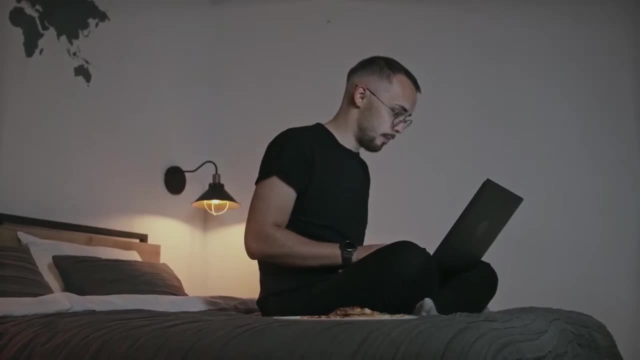 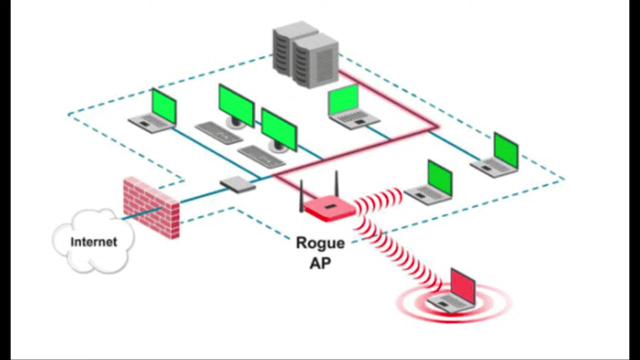 into installing malware on their devices or divulge sensitive information. The third is rogue access point. Devices with wireless cards usually try to automatically connect to the access point with the strongest signal. Attackers can set up their own wireless access points and trick nearby devices into joining their domain. 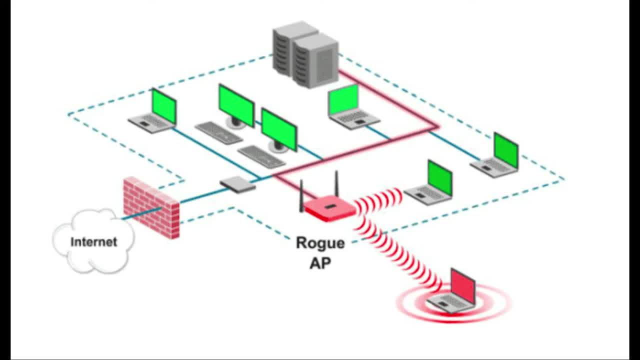 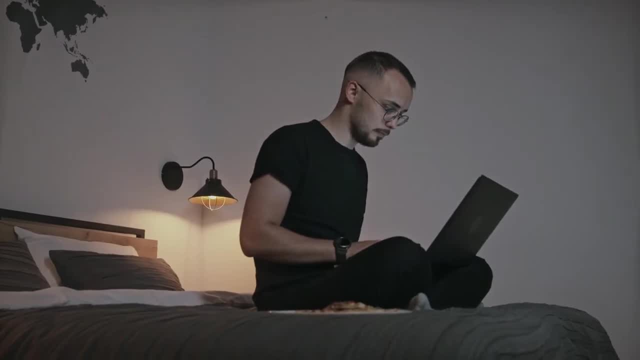 The third step is network traffic. All victims' network traffic can now be manipulated by attackers. This is dangerous because it doesn't even require the attacker to be on a trusted network. The attacker just needs enough physical distance- The last types of man-in-the-middle. 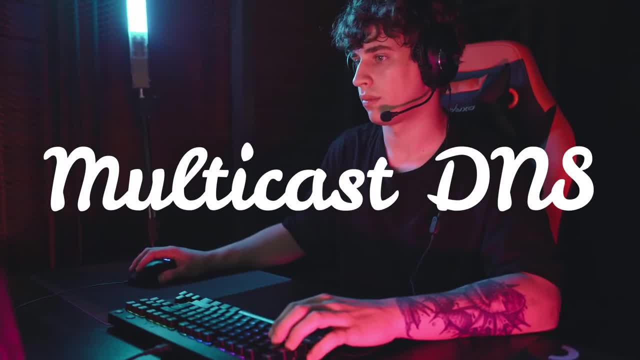 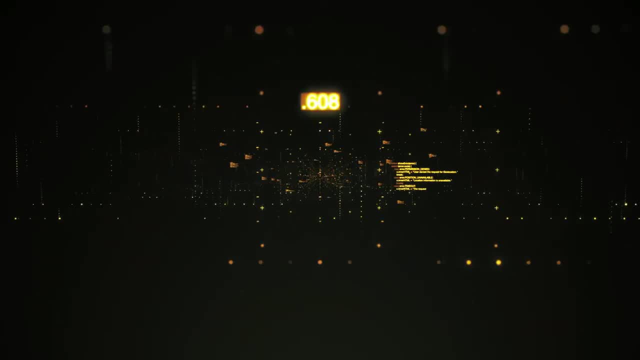 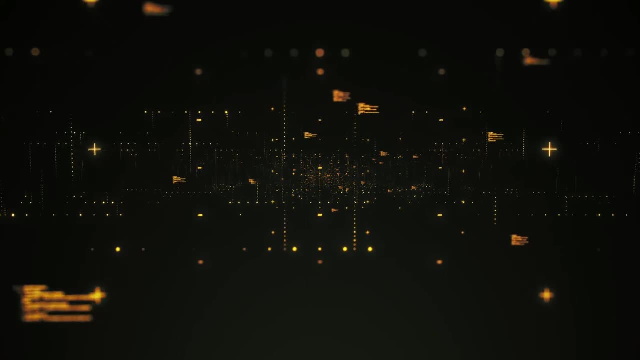 attack is MDNS. spoofing Multicast DNS is similar to DNS, but it's done on a local area network using broadcast-like address resolution protocol. This makes it a perfect target for spoofing, and spoofing The same resolution system is supposed to make the configuration of network. 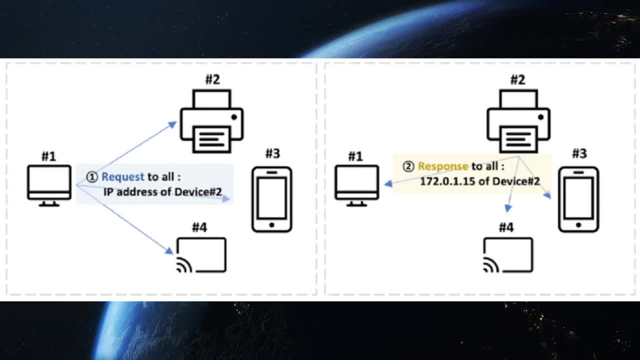 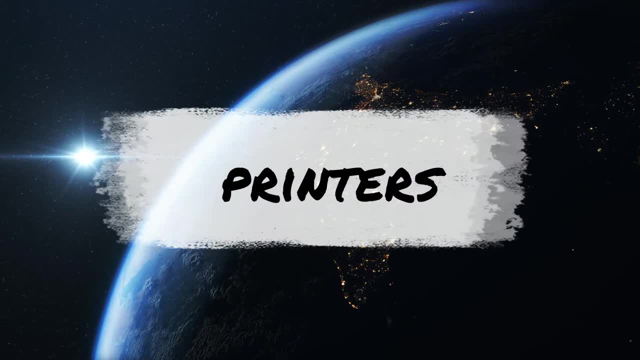 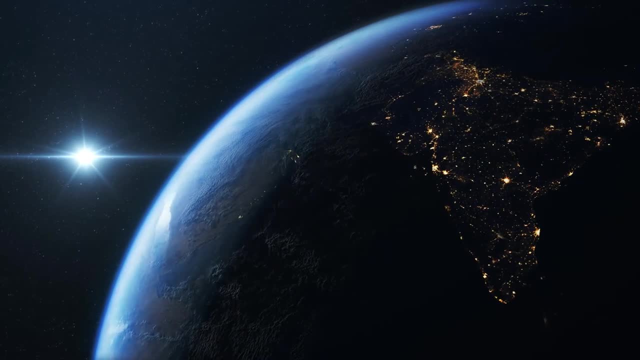 devices extremely simple. Users don't have to know exactly which addresses their devices should be communicating with. They let the system resolve it for them. Devices such as TVs, printers and entertainment systems make use of this protocol, since they are typically on trusted networks. When an app needs to know the address of a certain device, such as TV local, an attacker 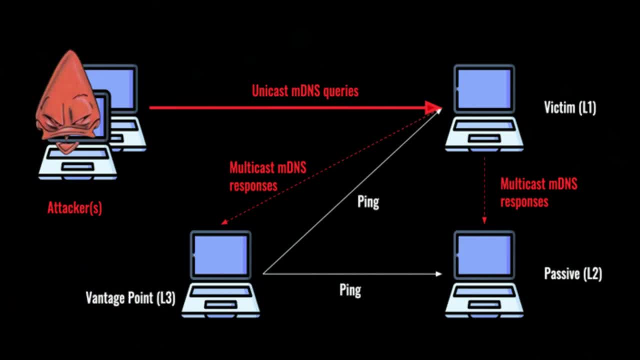 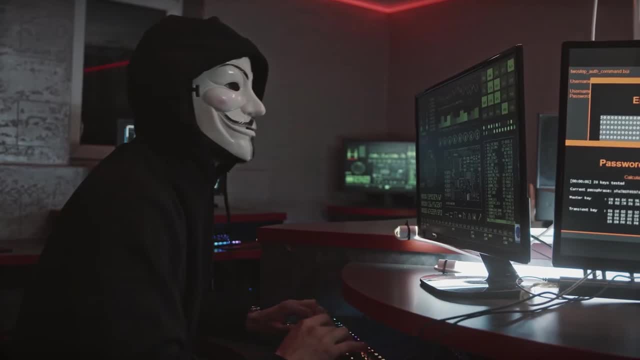 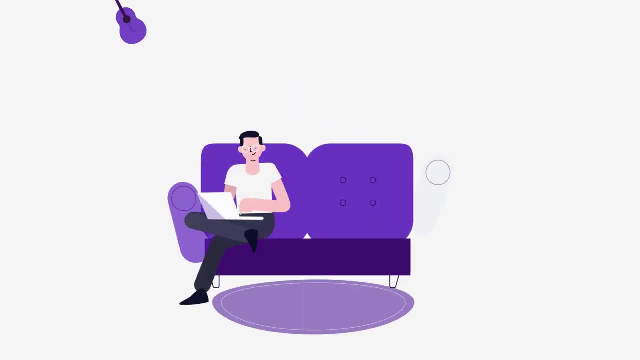 can easily respond to that request with fake data. An attacker can also respond to an address it has control over, Since devices keep a local cache of addresses. the victim will now see the attacker's device as trusted for a duration of time. Now let's look how to prevent man-in-the-middle attack. 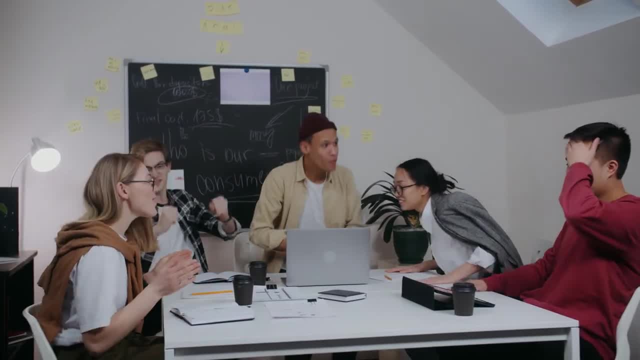 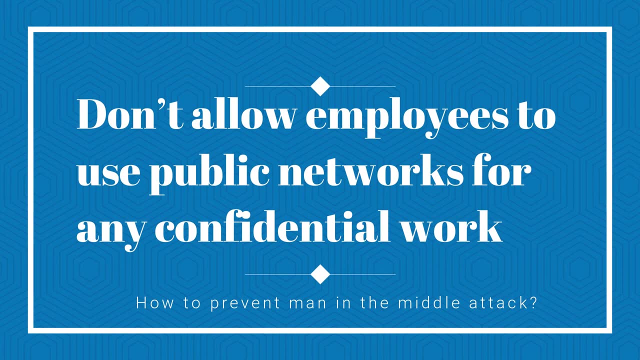 Here are a few steps businesses of any size can take to reduce man-in-the-middle attack risk. The first is: don't allow employees to use public networks for any confidential work. The next is: implement virtual private networks to secure connections from your business to online. 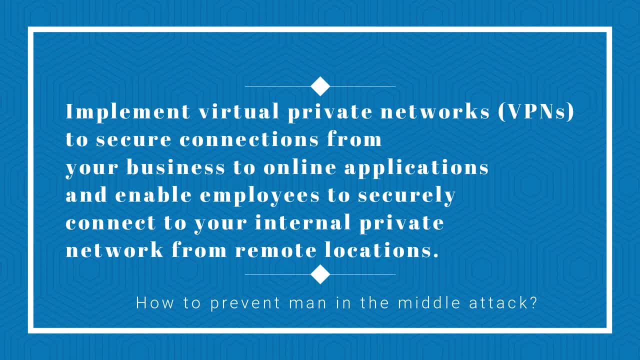 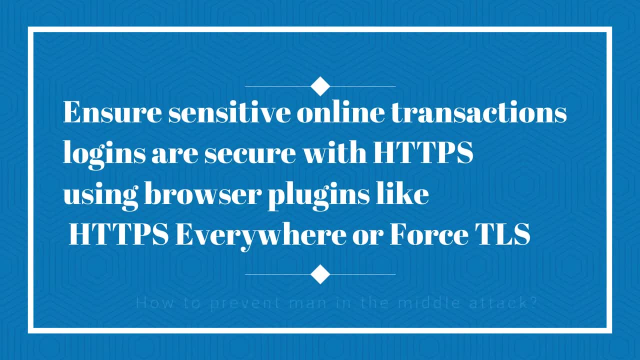 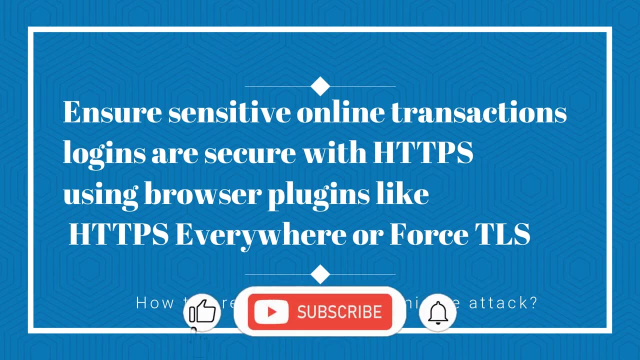 applications and enable employees to securely connect to your internal private network from remote locations. The next is ensure sensitive online transactions logins are secure with HTTPS using browser plug-ins like HTTPS Everywhere or ForceTLS. The next is use the latest version of high-security web browsers, such as Microsoft Word, Google Docs and Google Docs. The next is use the 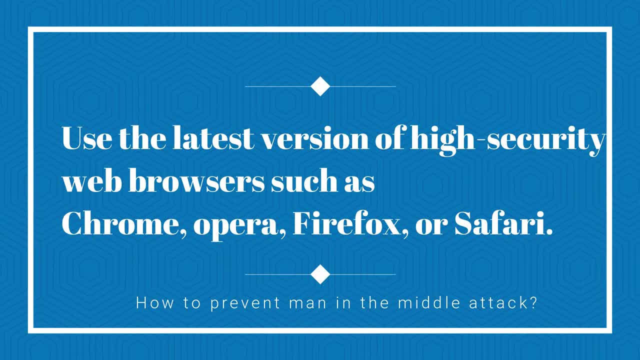 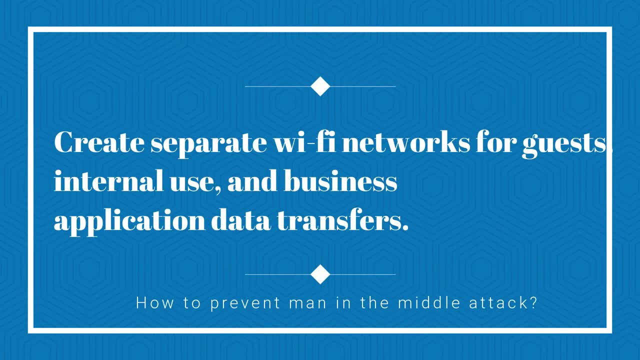 latest version of high-security web browsers, such as Microsoft Word, Google Docs and Google Docs such as Chrome, Opera, Firefox or Safari. The next is create separate Wi-Fi networks for guests, internal use and business application data transfers. The next is utilize authentication.